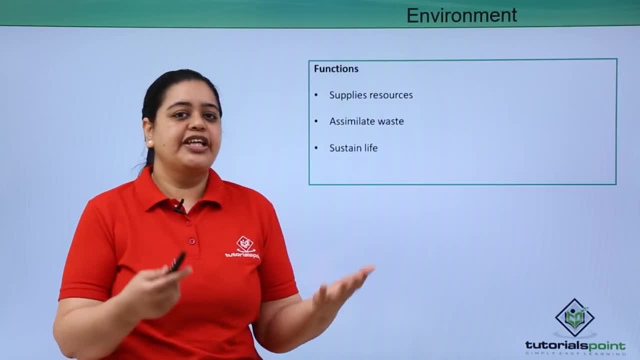 Now you would have heard about this thing, that honeybees. Now they are the most important, Important thing in case, if they all get extinct, the humans won't be able to survive for more than 7 days, The reason being because they help in pollination. 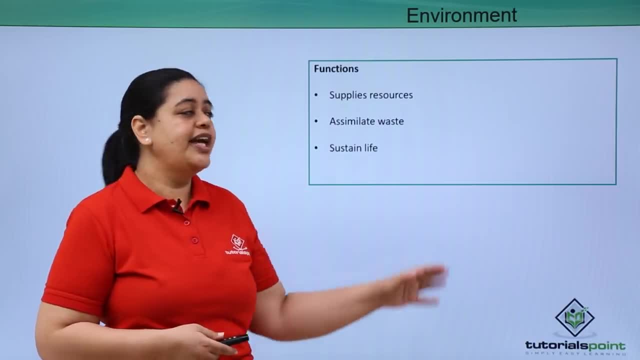 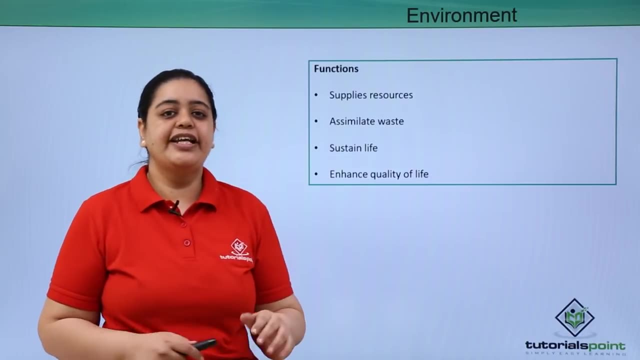 So, similarly, all these creatures play an important role, and it is the environment which is providing us Now. it enhances the quality of life because of the resources it is providing to us. Now let's understand the crisis as such we have in terms of environmental. 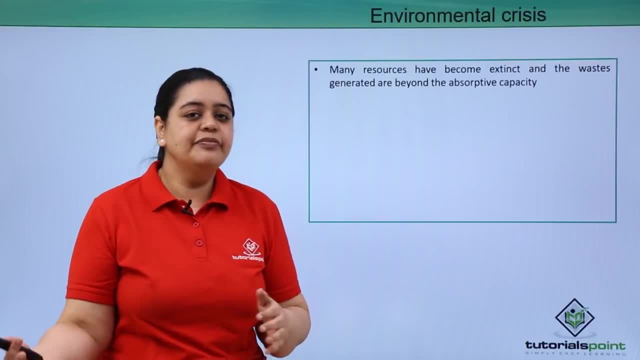 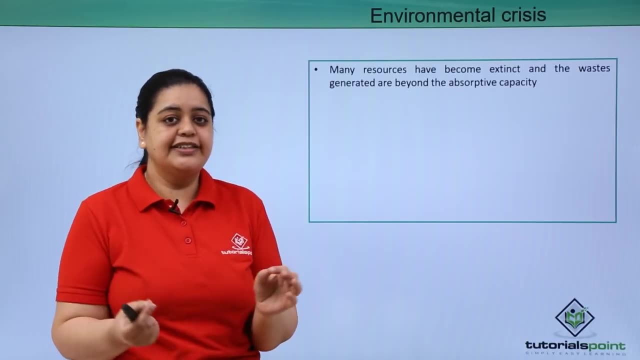 Now most of the resources have 2 hours Becoming extinct. they are going to become extinct or they are 2 hours becoming an extinct and the waste is which, that is, the wastages which are generated are beyond the absorptive capacity. Okay, 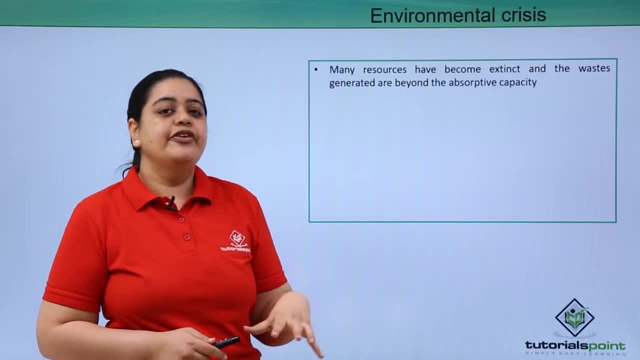 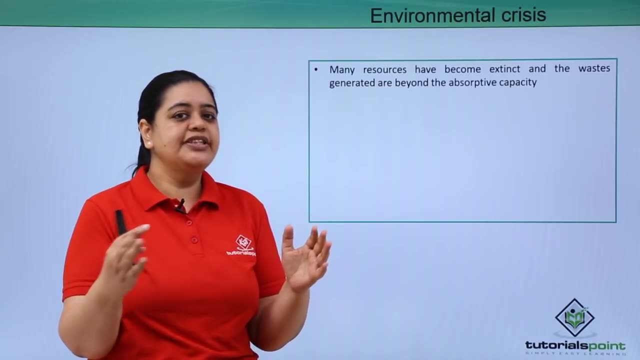 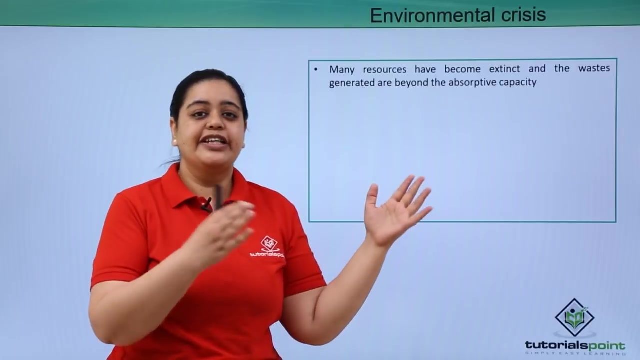 So what is happening out here is that we have utilized the resources so much that now we are on the brink of extinguishing those resources, that is, those resources becoming extinct, and then the wastages which are being generated. Now, in the earlier slide I told you it assimilate waste. 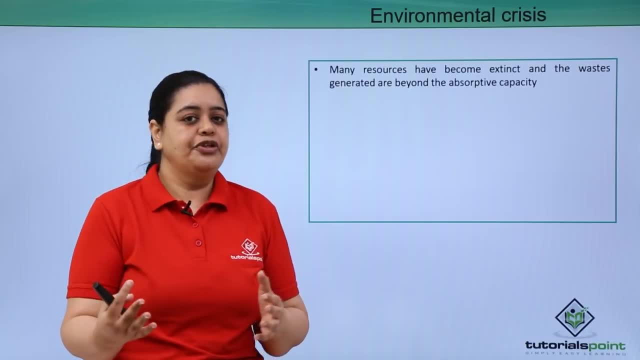 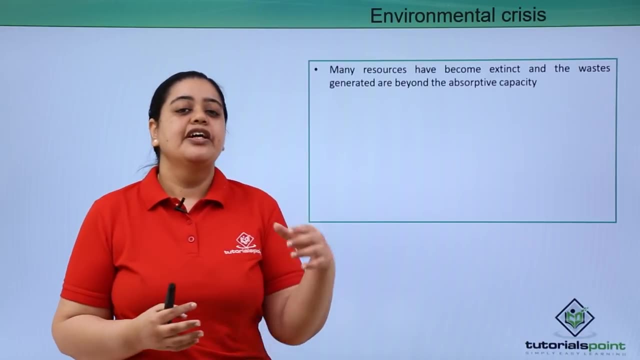 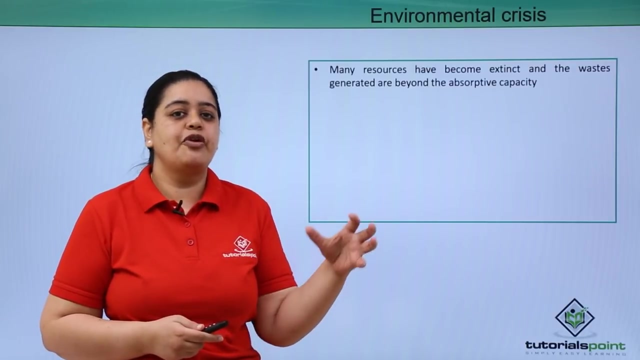 What is happening there? Whatever waste earlier we used to produce as humans, that mother nature used to recycle for it, but then we produce certain things, for example plastics and everything, and also the other waste which we are producing now. that waste is not being absorbed properly by the environment because the amount of that waste has increased. 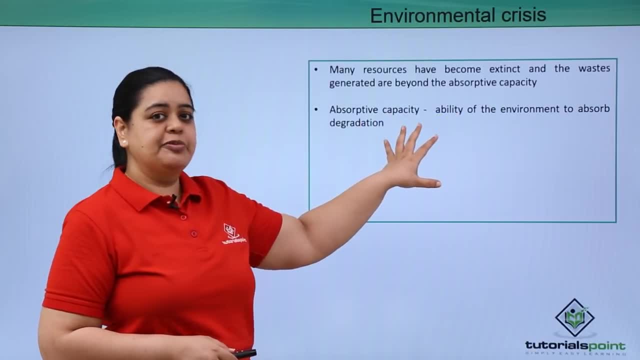 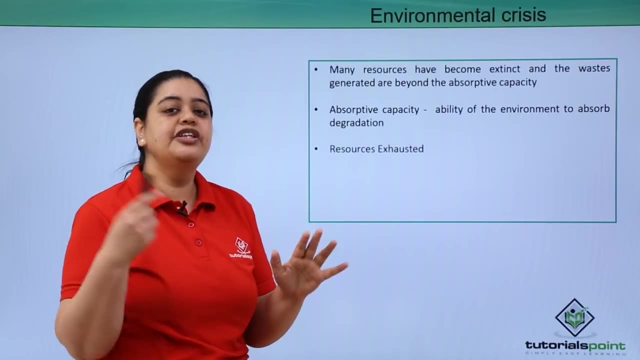 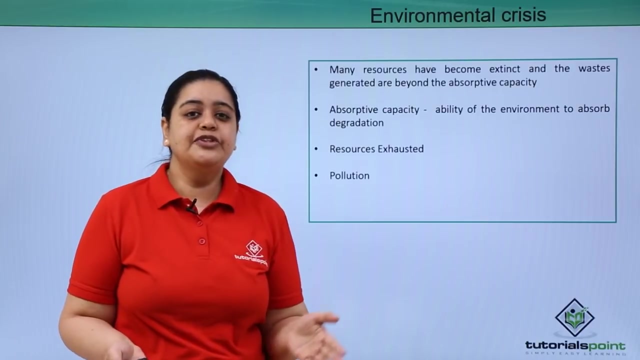 So see, absorb it Or just to give you the absorptive capacity is nothing but the ability of the environment to absorb degradation. So that has now reduced to a large extent. Now, again, the resources I already said have been exhausted. We are suffering most most important problem, which is pollution: air pollution, water pollution, noise pollution. 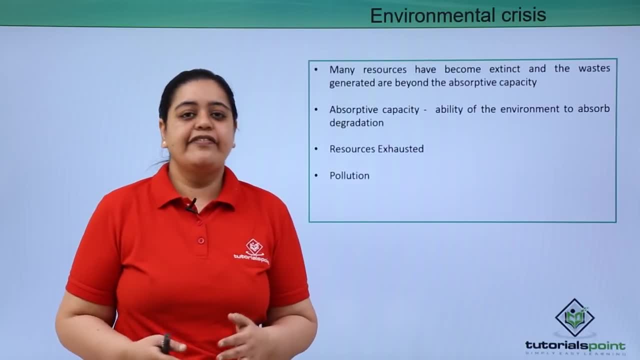 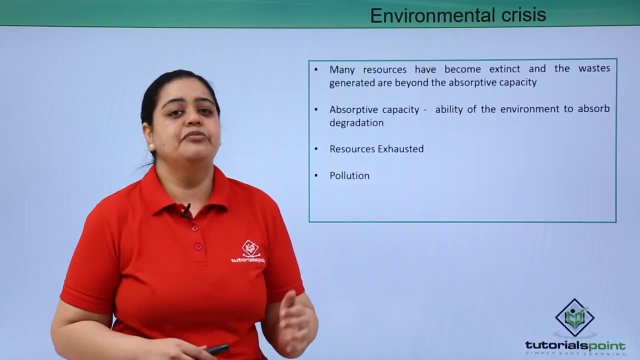 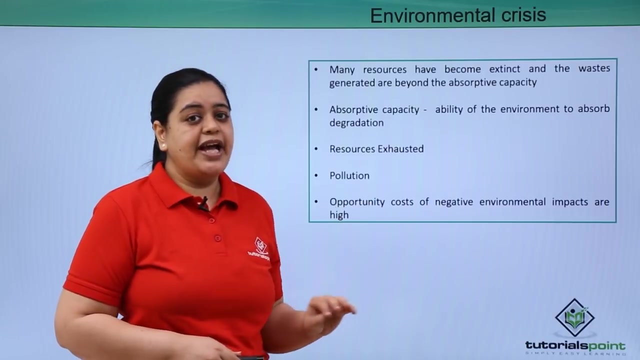 We have so many different kinds of pollution which are affecting our life, and it's not affecting our life only. it is affecting the marine life as such. It is affecting The life of the animals and the birds which are there Now. the opportunity cost of negative environment impacts are very high. 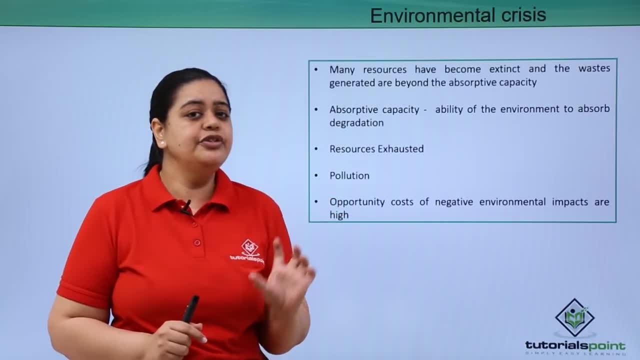 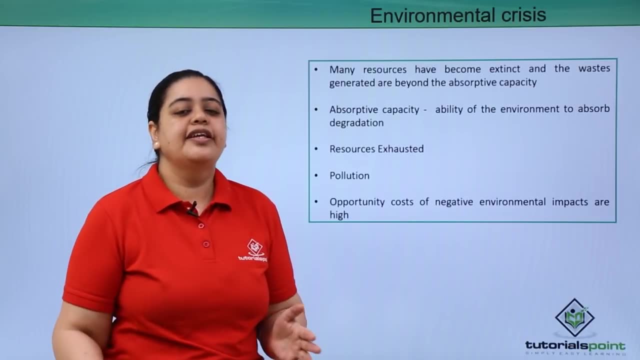 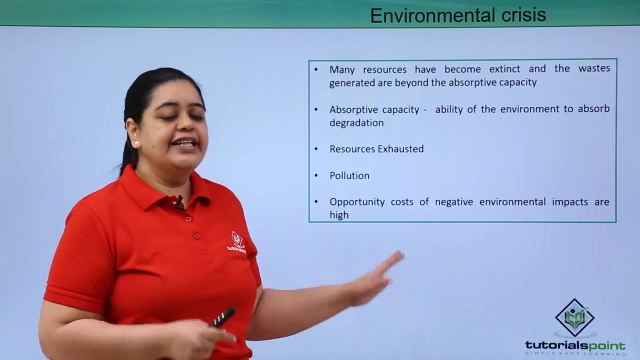 Now, I have been telling you water is very scarce. I told you that 1% of the water is the drinkable water. Now, if you're wasting that water and you're exhausting, you're not keeping proper storage of the water or you're not doing rainwater harvesting, then what is happening is you're creating more pollution. 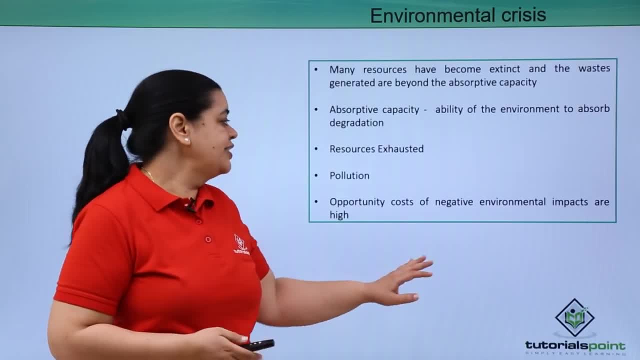 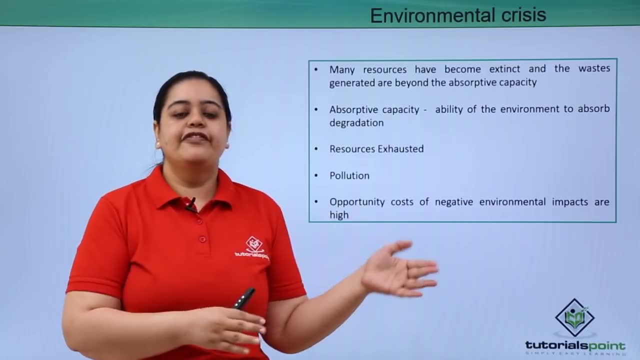 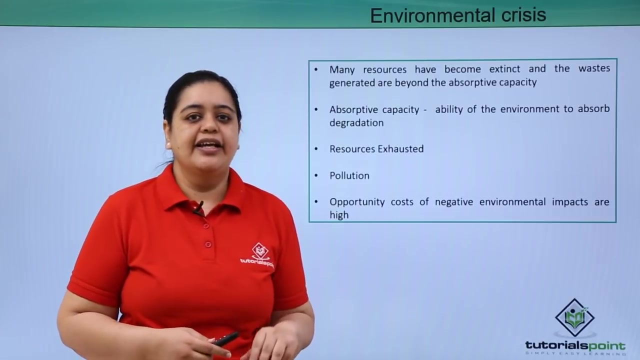 Apart from that, you're Waste, exhausting the resources, then there would be a negative environmental impact and then the opportunity cost would be very high. Example: if the water which is available for drinking is exhausted, if there's no water left and you have forced to depend on sea, then the desalinization process is very costly and it is not that easy to do it. 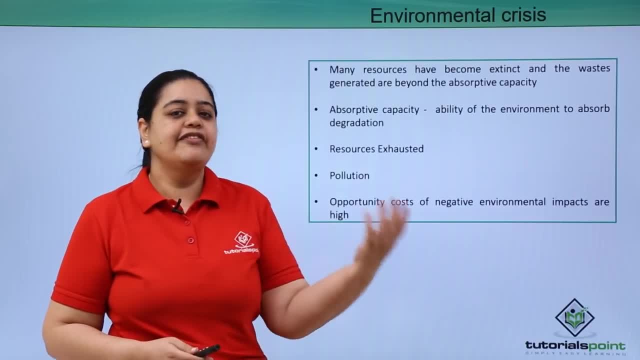 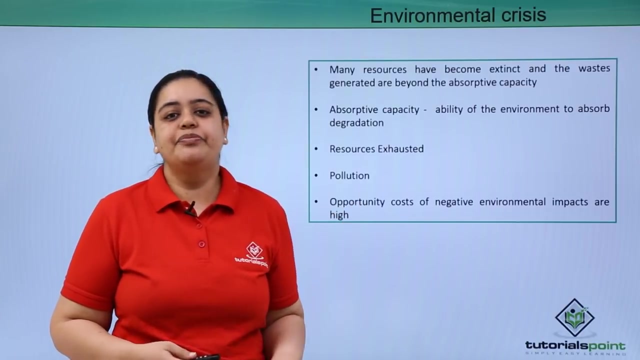 So again you're increasing your cost. Similarly, if your resources get exhausted, then you would have to Search for alternative ways, which would be very costly. again, the pollution which you're creating in the environment that is impacting the health of the people, so it would create a lot of problems even there. so that is the reason it is said that opportunity cost of negative environmental impact is very high. 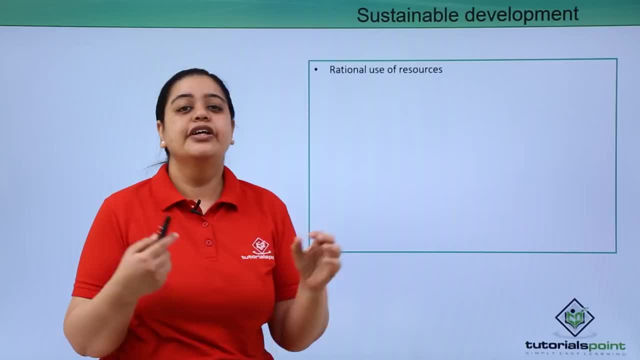 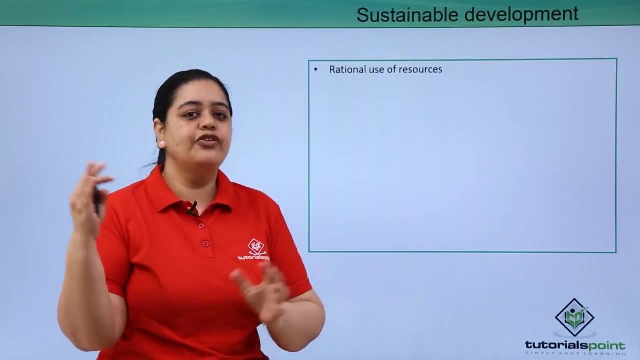 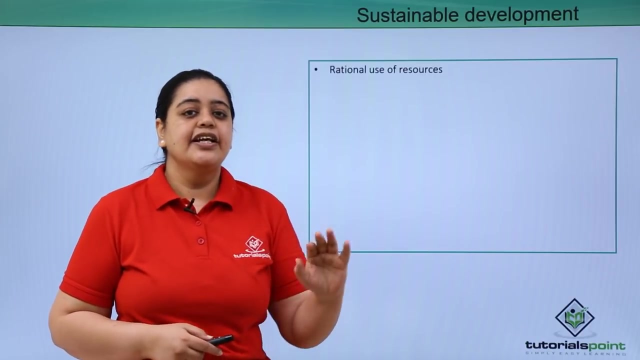 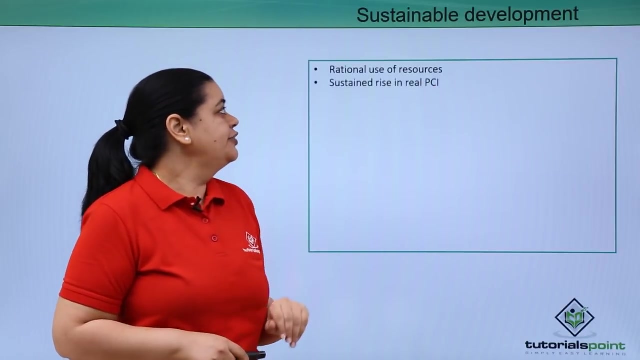 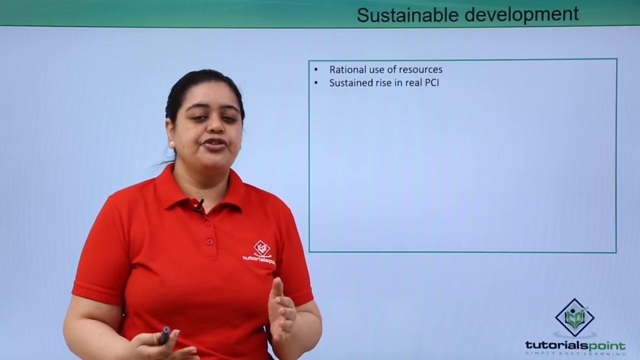 Now let's understand further. You need to For a sustainable development, that is, a development Which Can be sustained over a period of time, which is there for a number of years. then you need to use your resources in a rational manner. avoid wastages, use the resources as in a proper, judicial, planned manner. as such, you need to have a sustained rise in the real per capita income, so you have to keep on ensuring, as a country, that your per capita income is rising now. 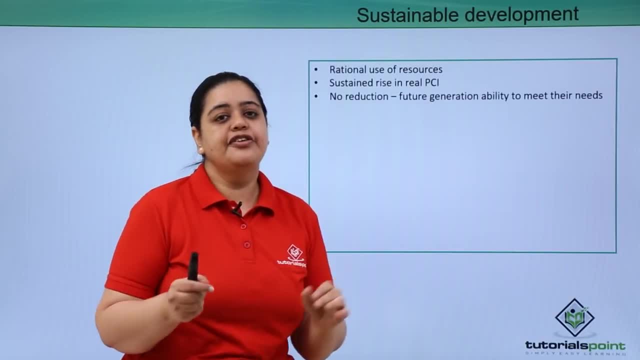 If you're not reducing your dependency on resources or if you're wasting it, then future generation would not be able to meet their demands. See, as of today, if I see, the country as such has a huge amount of population. we have more than a billion. 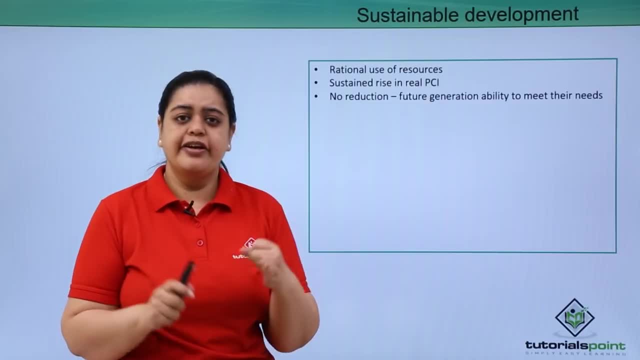 Now we have so many people who require air, who require water- and I'm just talking about the basic things- and food. If you keep on wasting the land- for example, if you Don't Too much of waste on the sodded land- then the land gets useless. 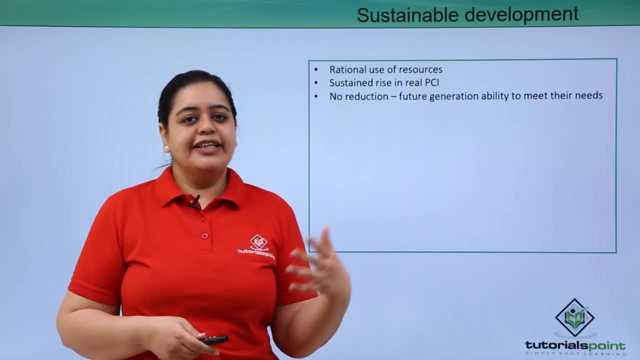 It is not used, or cannot be used for agriculture. Similarly, air pollution, the more the air pollution you would have seen. nowadays, most of the children are allergic to dust. We keep on sneezing when the moment we are out. there are so many diseases which keep on happening. 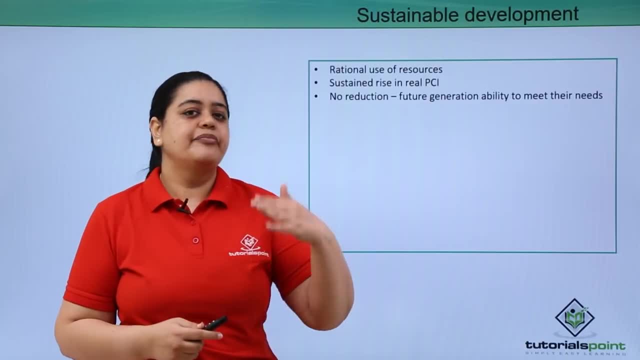 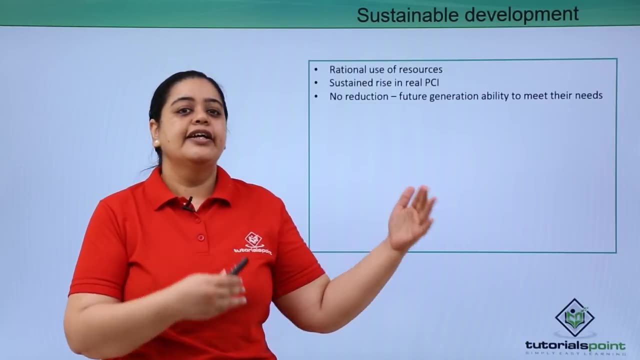 The immune system is already reduced compared to the people, the older people in your house. you would have seen your grandfather, or you would have seen your mother and father. Comparatively, they are more better in terms of health. Now why the health is deteriorating because of the pollution effects. 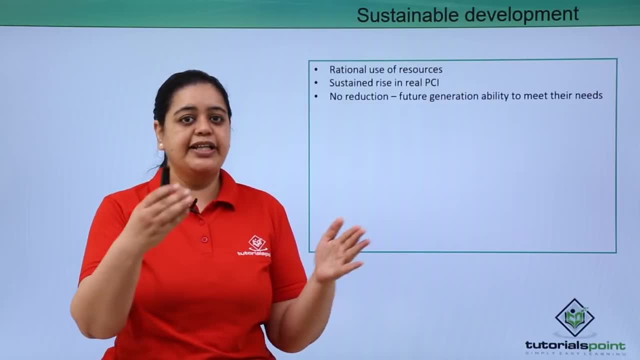 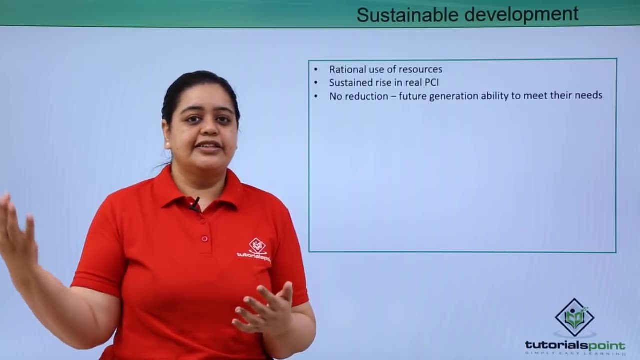 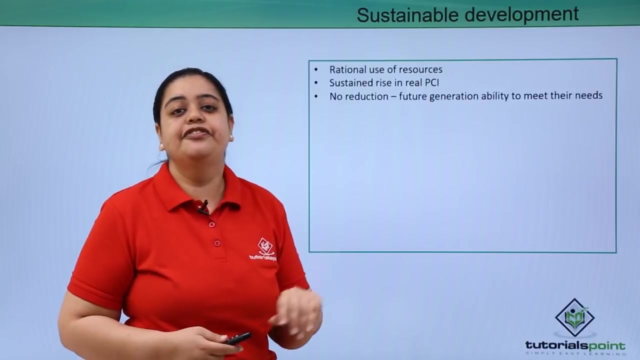 Do we have better access to drinking water? Yes, But then how far that water can be used? because we are not doing any water harvesting, We are not using solar, sun energy- which can be- which is available for free, So all these things are impacting and hence the chances are that the future generation will not be able to meet their needs is quite a possibility. So all these things are impacting and hence the chances are that the future generation will not be able to meet their needs is quite a possibility. So all these things are impacting and hence the chances are that the future generation will not be able to meet their needs is quite a possibility. 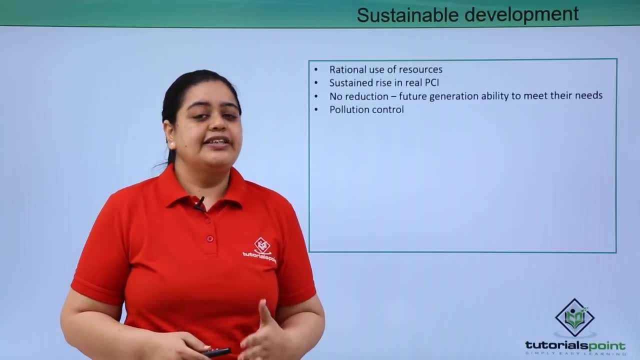 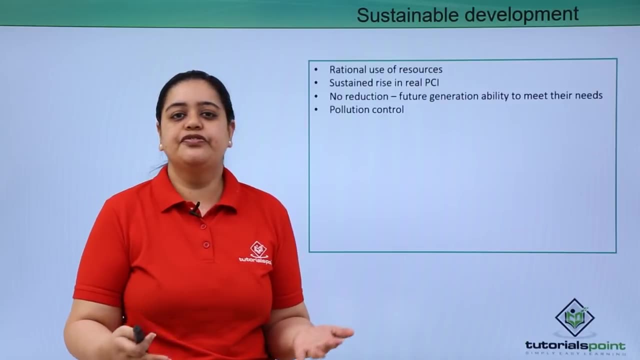 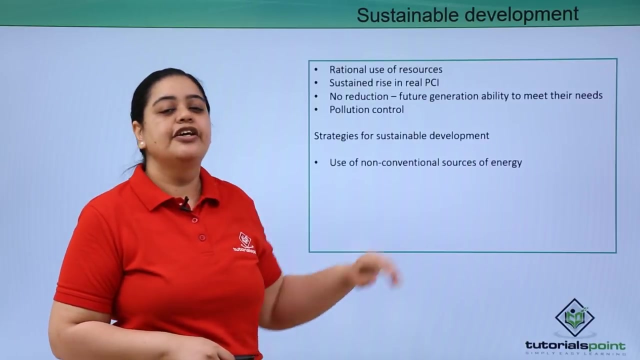 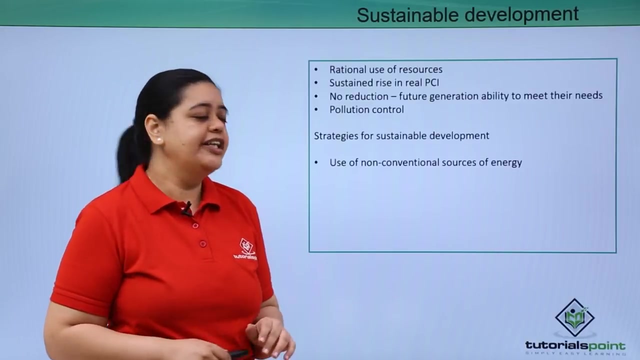 Pollution control. we need to control the pollution, Otherwise the environment will degrade further and the place that is the country as such would not remain a place where people can live. Now what are the strategies for sustainable development? You should use non conventional source of energy, which I explained you earlier, like your solar energy, tidal energy or wind energy. 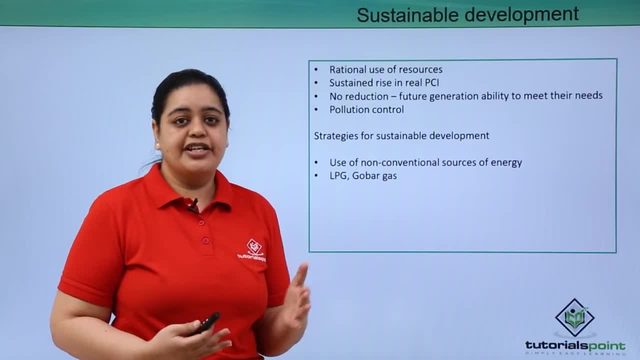 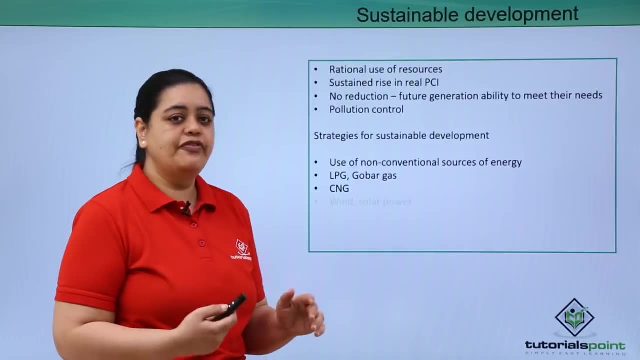 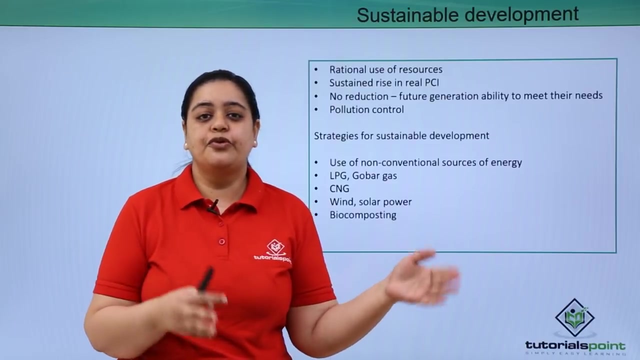 Now, use of LPG should be preferred, goba gas should be preferred now, in terms of CNG, it is more preferred compared to use of any other form of petrol. then wind, solar power, as i already said, biocomposting instead of depending more on. 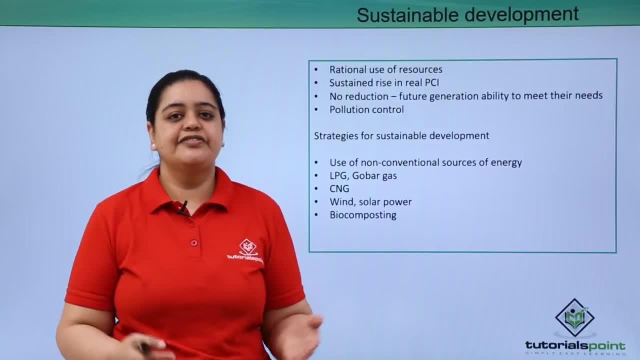 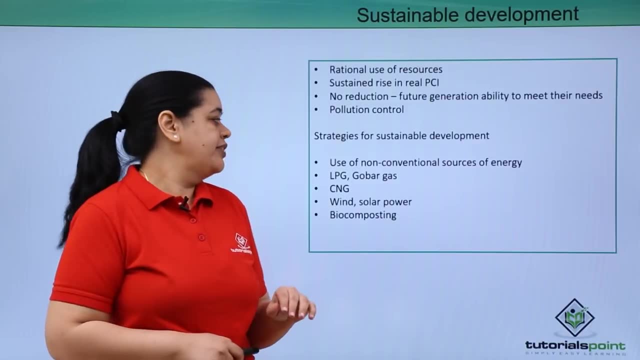 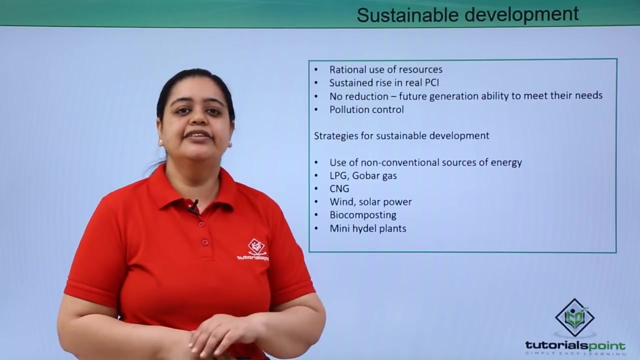 fertilizers. use of biocomposting, wherein the waste which is being thrown out from every household that can be utilized in a better and a proper manner. you should also be using mini hydel plants, which helps you in sustaining the environment. then comes your biopest. what is biopest? wherein 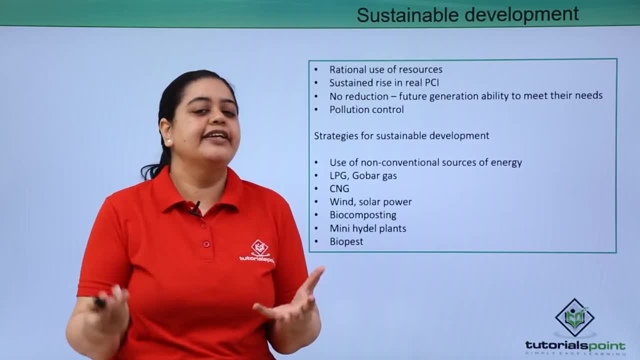 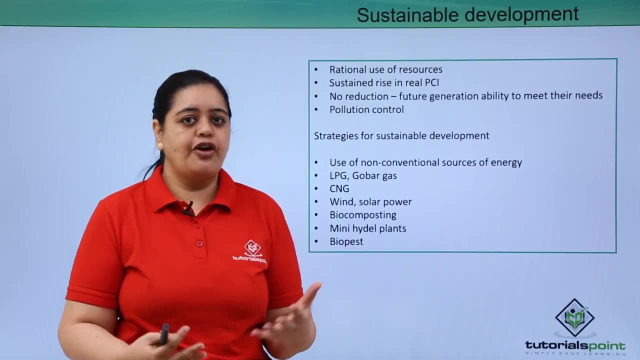 you are using the. instead of pesticides, you are using biopest, like the natural pesticides which can help in fighting the attacks which happen on crop. that is, you can also use biopest, which can help in fighting the attacks which happen on crop, the problems which we face when you are growing the crop. this we generally use pesticides for. 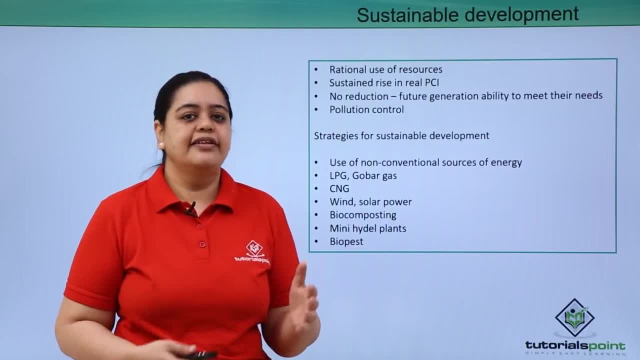 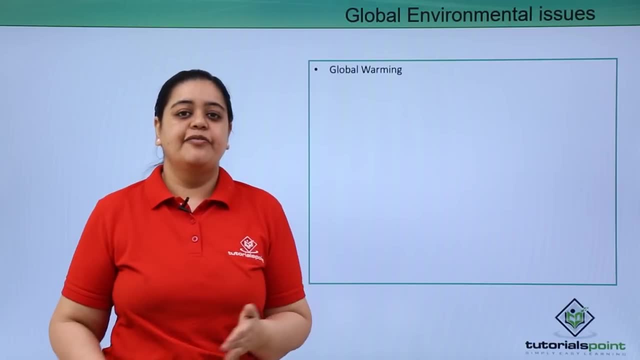 that, instead of that, use of biopesticides is recommended. now, next comes your global environmental issues. global warming is the most important factor or problem faced by the world today. we all know every year you would have seen your city getting more, warmer and warmer. the place you are living is becoming more warm and that is creating tons of problem in the 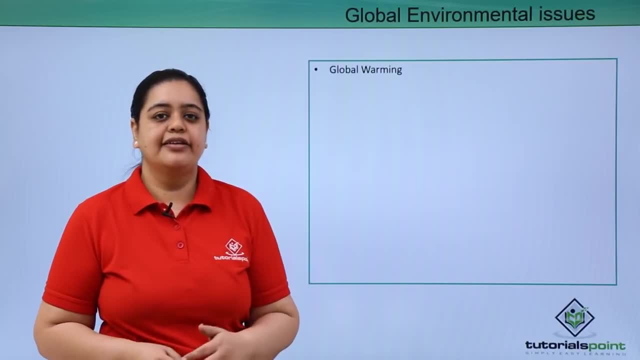 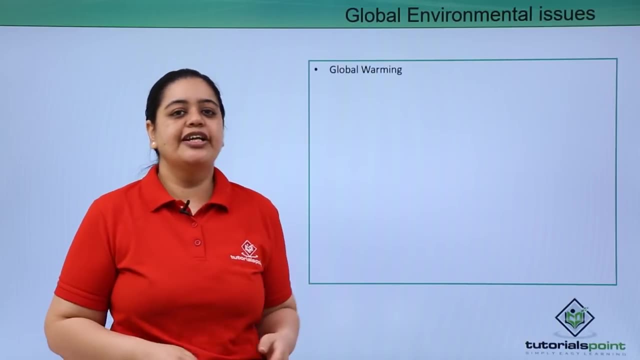 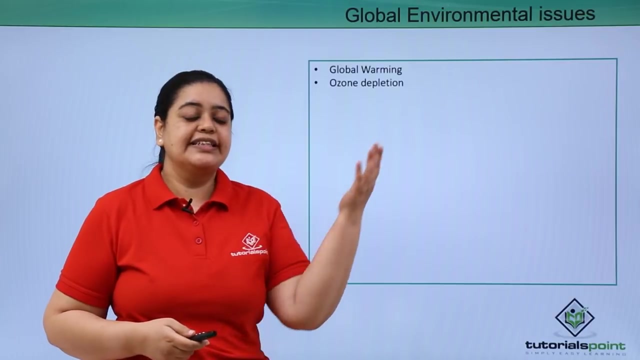 world globally as such, and if you see, in terms of countries committing to better environment, the commitment is very less. we are still struggling on those parts. there is a ozone depletion. you would have seen that for protecting ourselves from the Sun it is necessary we have that ozone. 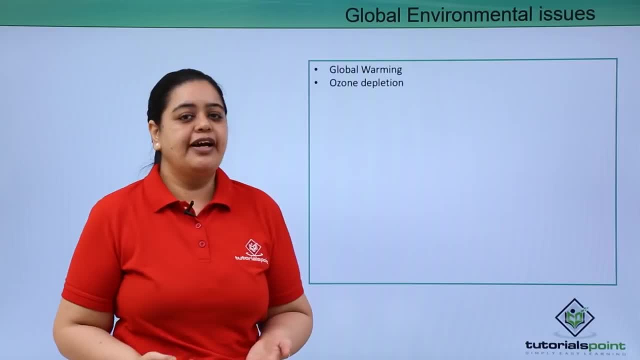 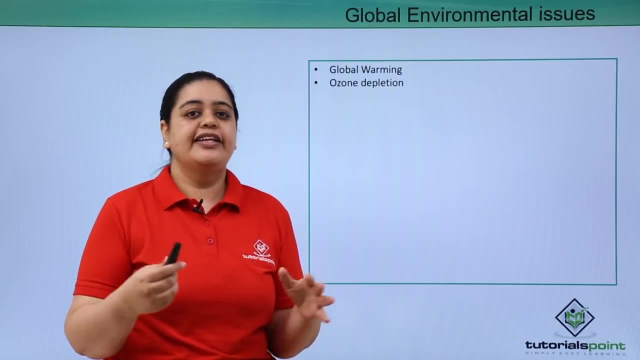 layer and that layer is now depleting. ozone layer is coming down the layers. we have seen lot many parts which have seen that depletion and hence what will happen if there is a study which was being made and it was published in the- it had come on Discovery Channel- that after few 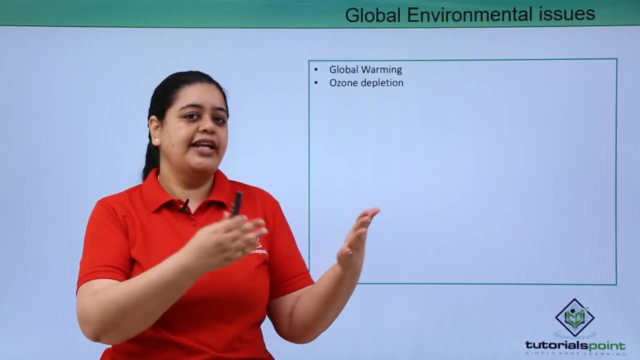 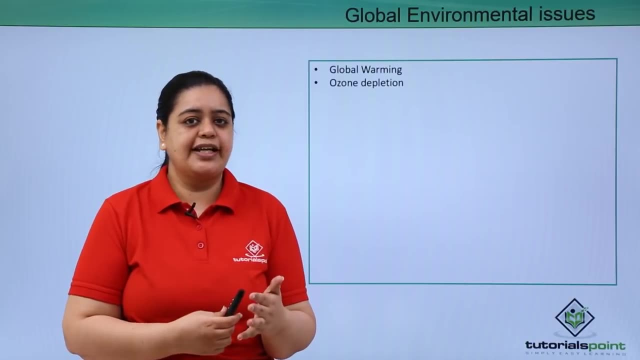 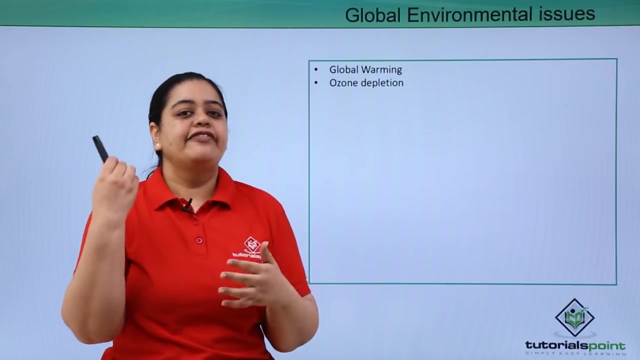 years, man as such would be like right now- we are on a fairer side- or, if I have to see, the skin would be totally damaged by Sun. because of this depletion and the impact of Sun and because of this warming which is happening, the global warming, in fact, we humans would now have, in coming years, red eyes. 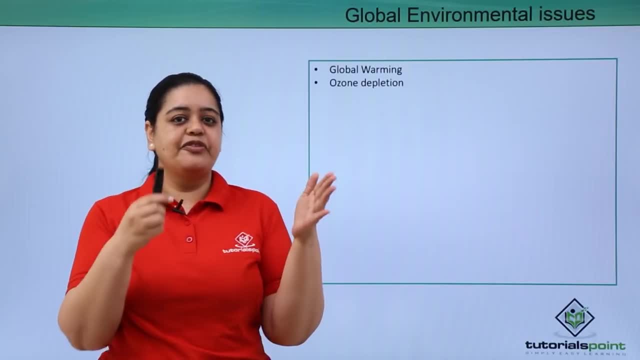 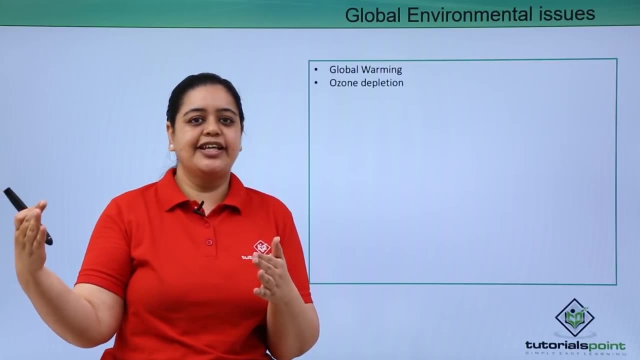 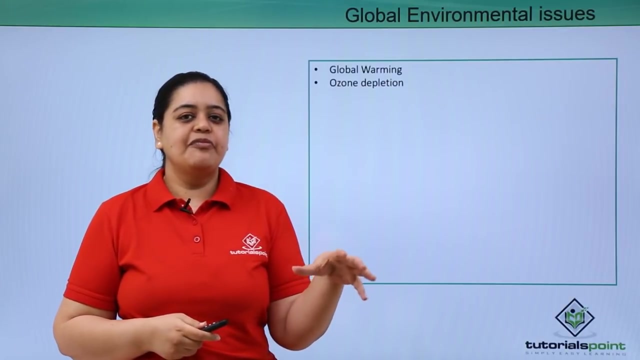 because of the damage which has been caused by Sun. so we would be growing to a climate which would be so hot that naturally the bodies will get adjusted there, but then the impact would be everyone would be having those red eyes. you can search that or more to get more information, but this was 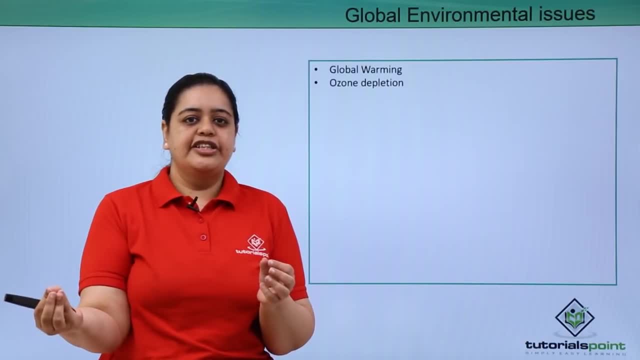 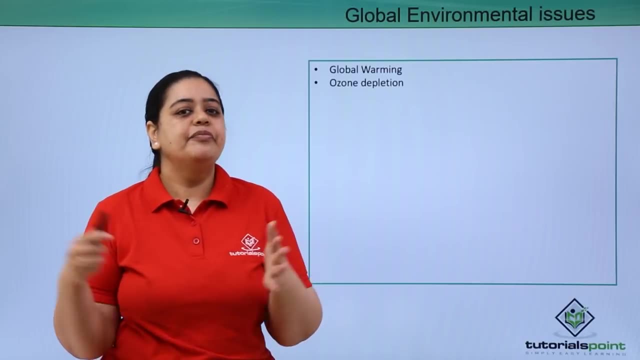 some kind of research which was being done and it was being told that, because of the rate at which the global warming is happening in, the temperatures are rising. pretty soon humans are going to suffer and this is the impact which we are going to have on our bodies. 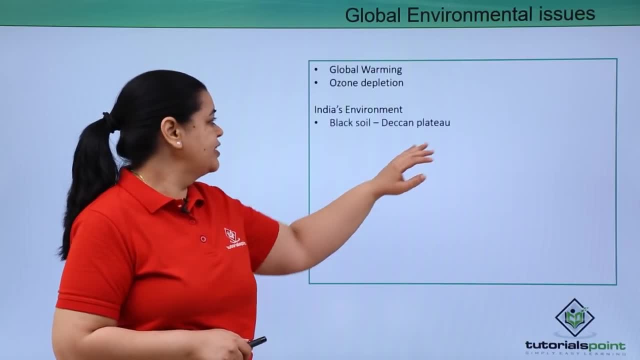 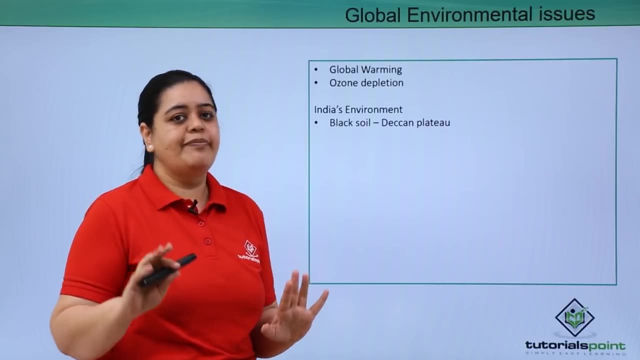 now let's see what is India's environment. see, we have a very beautiful environment when it comes to the soil pattern. we have a very beautiful soil pattern. we have different regions having different kind of soils. you would, if you would have traveled in India, you would have seen this. 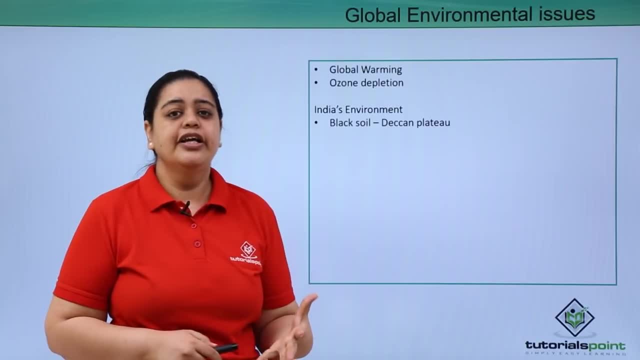 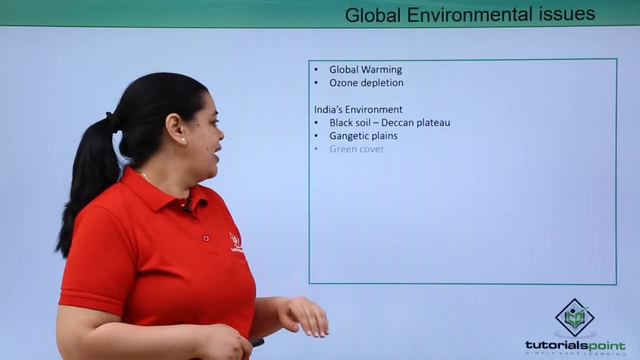 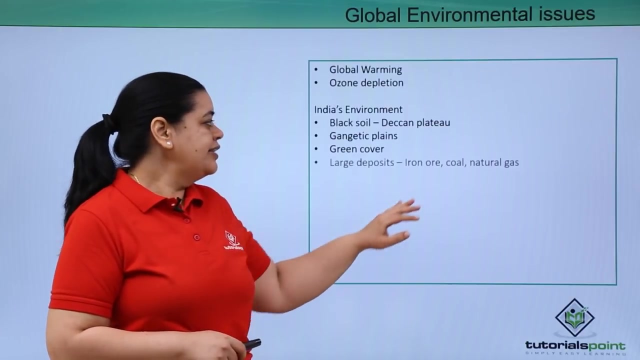 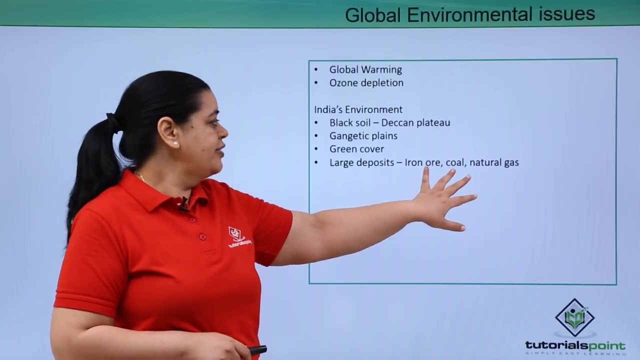 Deccan plateau, having the black soil, which is considered very good in terms of agriculture. then you have the gangetic plains. now these are also very fertile plains. as such, we have the green cover, which helps in protecting ourselves from the environmental damages. now, in terms of large deposits, we have huge resources in terms of iron ore, coal and natural. 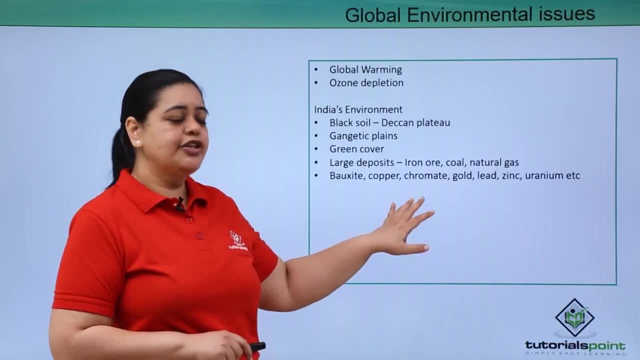 gases in the country. we also have bauxite, copper, chromate gold, lead, zinc and uranium, so we have a lot of resources in terms of iron ore, coal and natural gases in the country. we also have bauxite, copper, chromate gold, lead, zinc and uranium, so 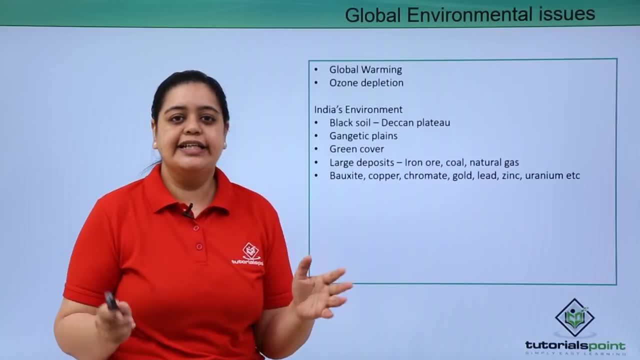 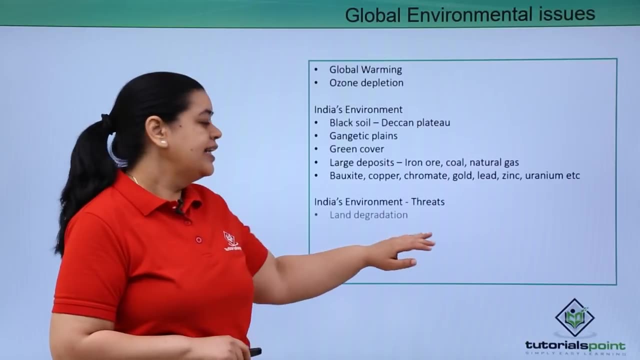 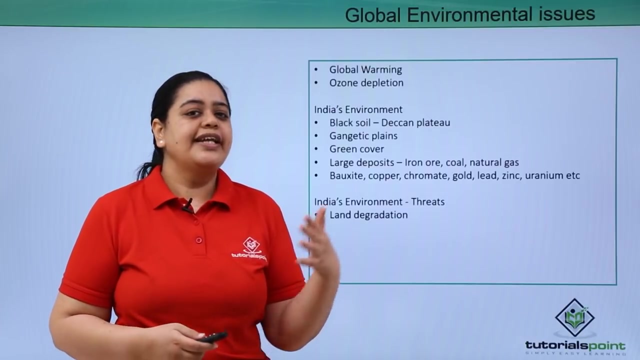 gold, lead zinc and uranium are also there. in terms of resources which we have. as an environment, however, the threats we are facing is land degradation, too much of wastage which we are generating as each of the household that is causing too much of degradation and the land. 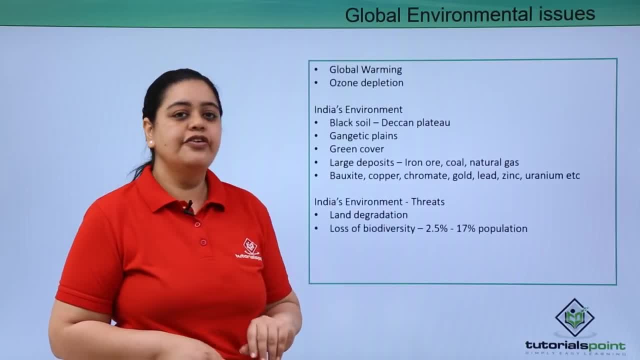 fertility is decreasing. there has been loss of biodiversity, so the loss has been approximately 2.75%, that is, 17% of the population being affected. we have air pollution. every city you go, even in tier 1, tier 2 cities, you have air pollution. then there is a problem of fresh water management. 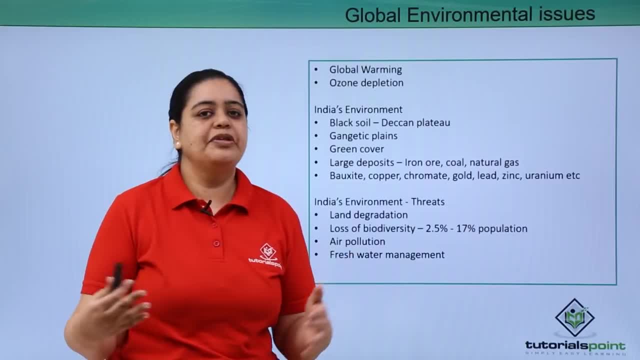 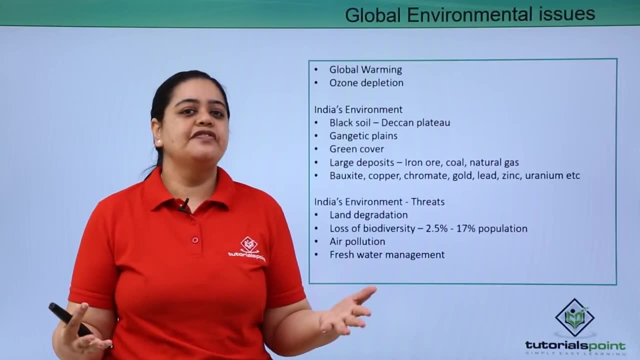 no doubt. we saw that 94 percent people have access to safe drinking water, but then we do not have much fresh water management. we all, most of the states, are fighting in terms of water. everyone has the scarcity of water, which isitos this are so difficult, and I think this is thelessness with respect to the water. there is a problem in the system we have, especially we just staying in the system. we have no water because the water is precious in terms of anotherім. 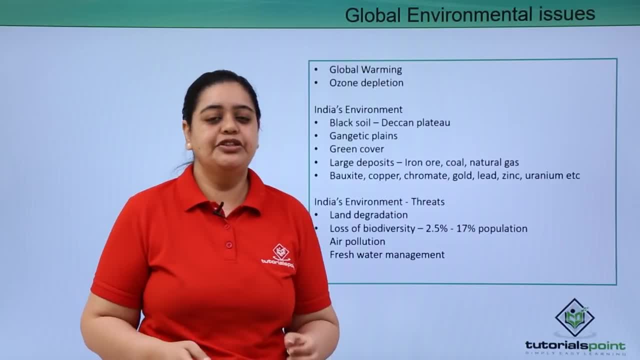 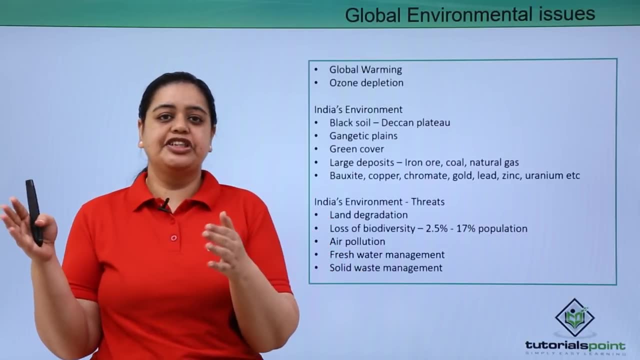 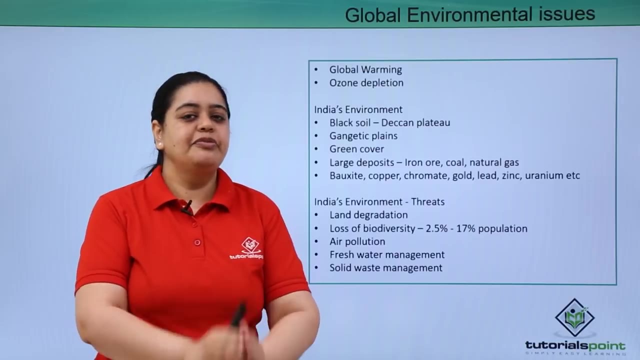 everyone has the scarcity of water, which has to be looked into it asap now. the last one is the solid waste management. this waste which is getting dumped on the grounds, that has to be managed in a more, better manner. otherwise it would be like you would be seeing all these dumps being lying.